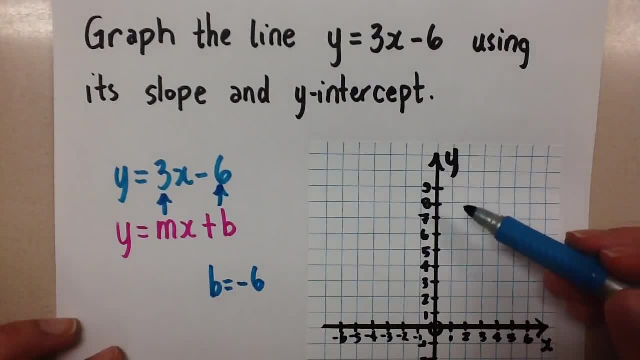 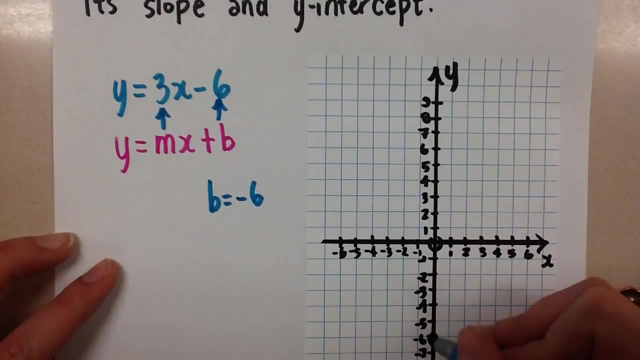 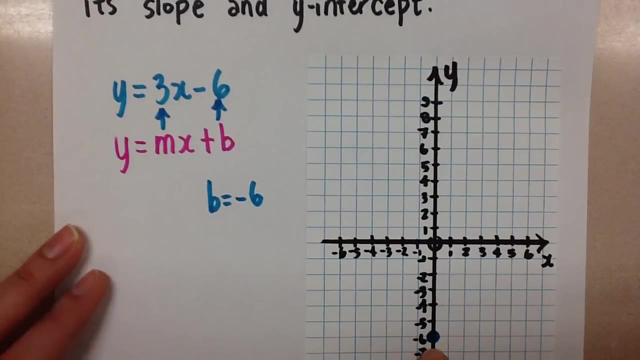 on the y-axis, the line will cross at negative 6.. So let's go down here On the grid and put a point at y equals negative 6.. So there's our y-intercept, that b value. The line has to cross there on the graph. 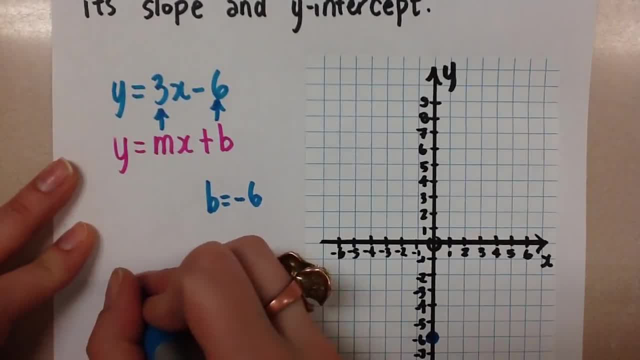 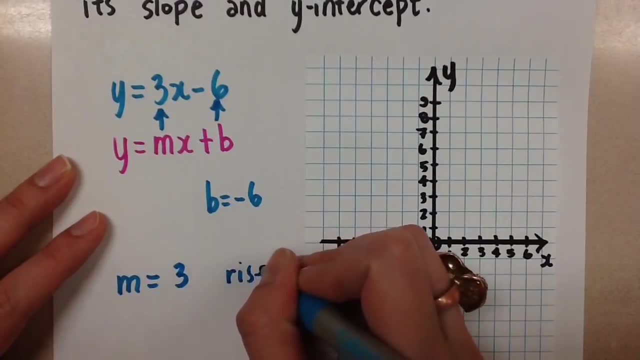 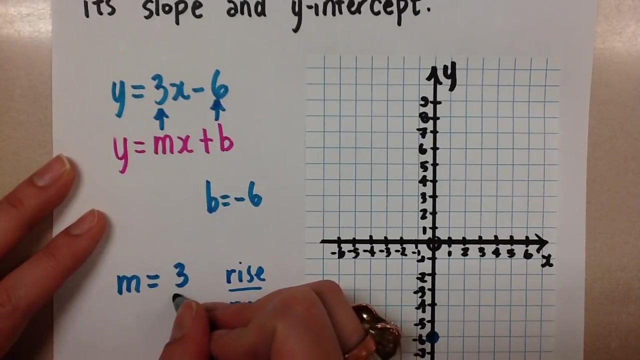 Now let's look at the slope. The slope from the equation is positive 3.. And if you remember, the equation for slope is rise over run. So we have the 3 here. We're going to write that into a fraction by doing over 1 like this. This doesn't change. 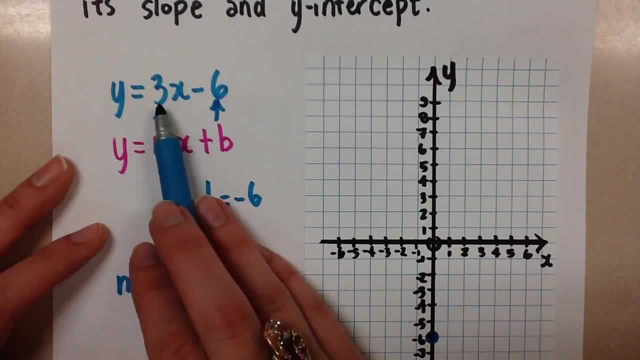 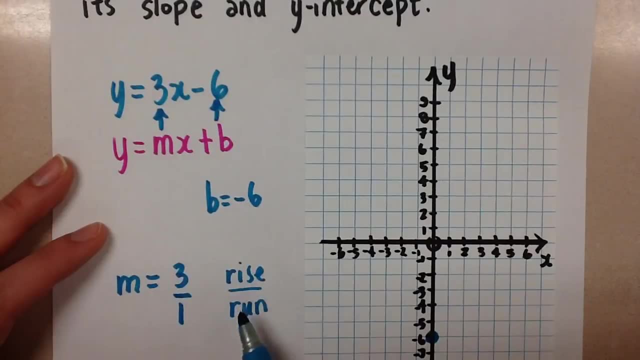 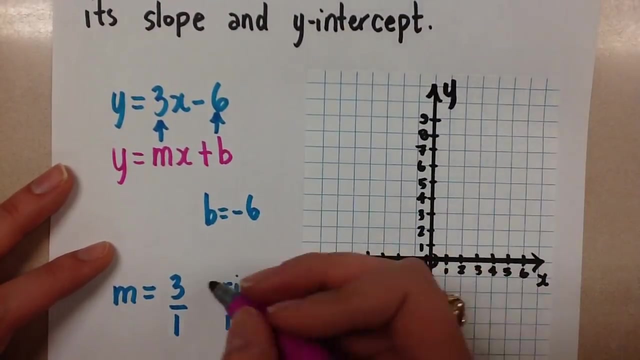 the value. If you already had a fraction for your slope, then you would use the numerator of the fraction for the rise and the denominator for the run. But since we didn't have one, we're going to create that denominator. and now we see that the rise is positive 3 and. 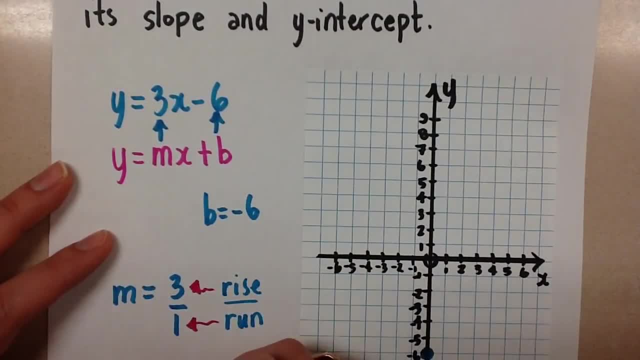 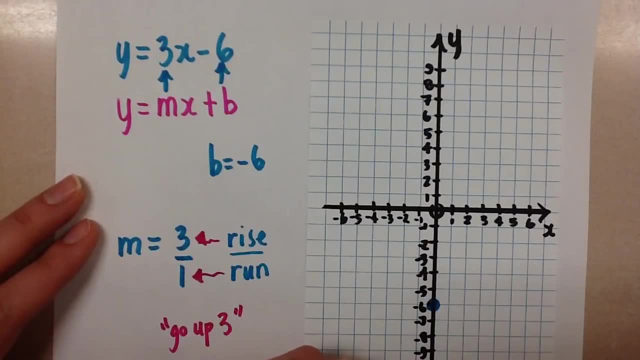 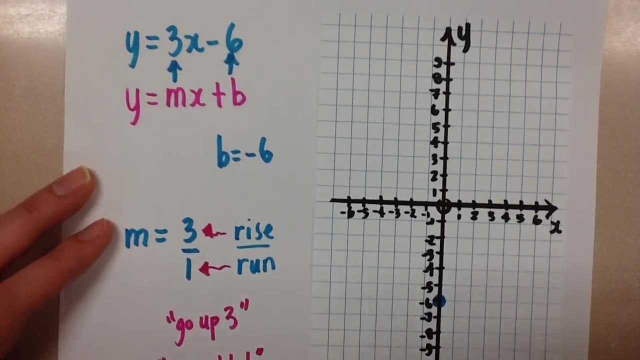 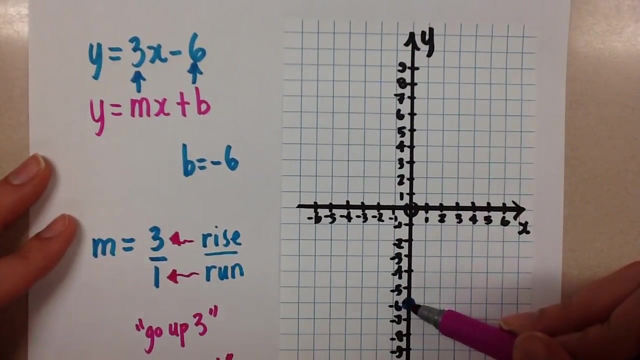 the run is positive: 1.. Go up: 3 for the rise and go right: 1 for the run. So we're going to go over to the y-intercept that we started on the graph here and we're going to do exactly what the rise tells us. 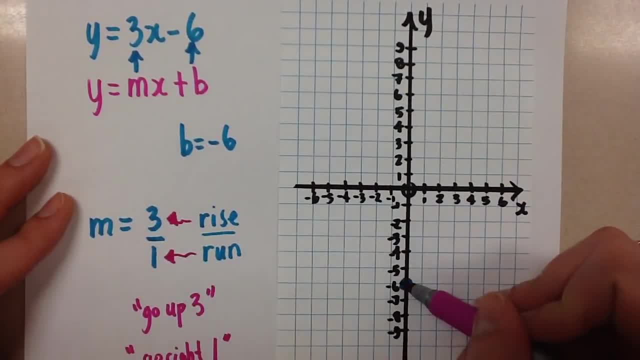 Go up 3, because it was positive 3.. So from here, I'm going to count 1,, 2,, 3 up, and then I'm going to do what the run says, which is: go right 1,, right 1.. 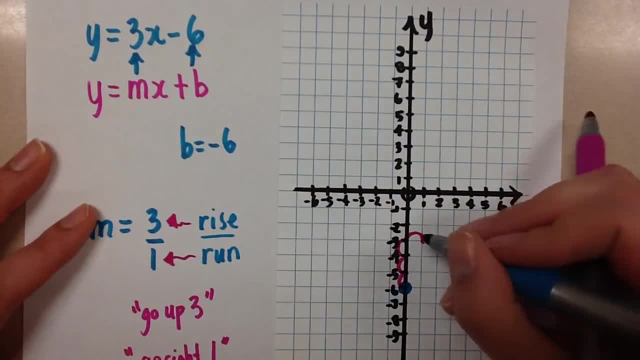 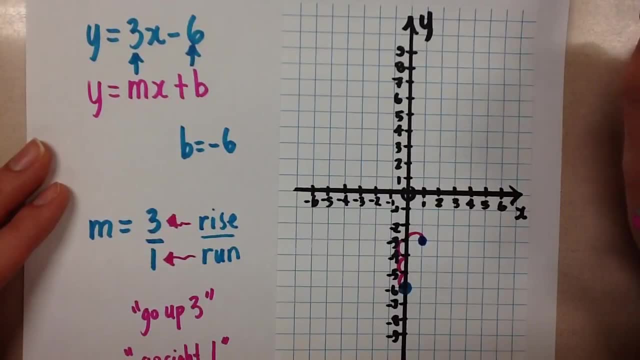 Right, there is my new point for this line. So now we have two points, We can draw a line through those two points and that's the line for this equation. I can also keep going with my slope. if I want more points Again, I would go up 3, 1,, 2, 3, and right, 1, and right. there would be another point. 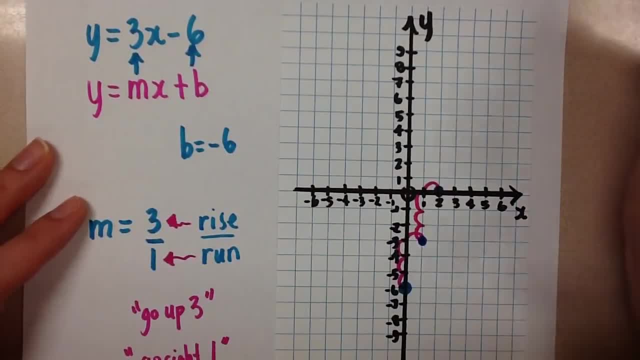 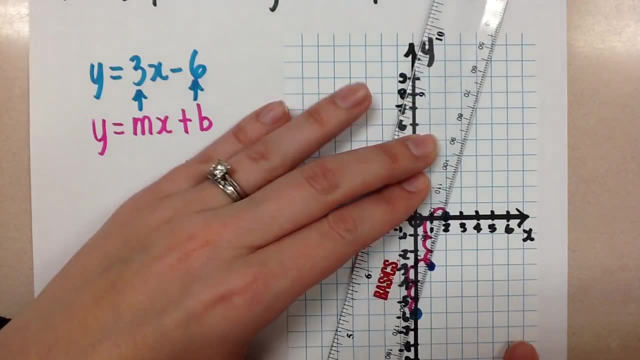 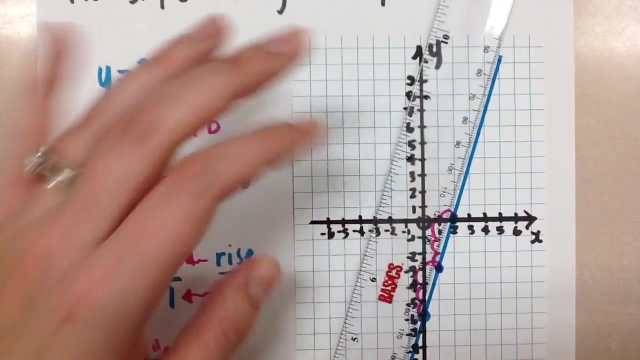 And I can keep doing this until I get as many points as I want, but really you only need two points to draw a line. So we take our ruler now and we try to line these up as best as possible. Draw your line all the way across the grid. nice and long. 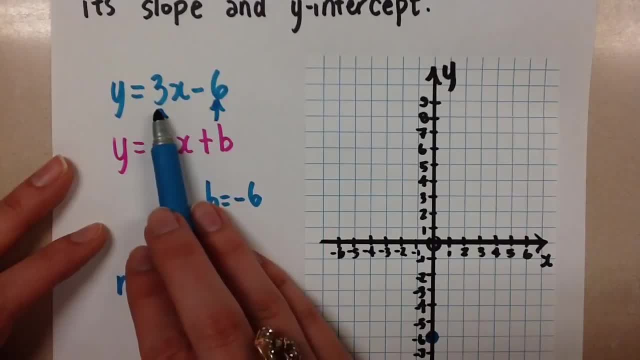 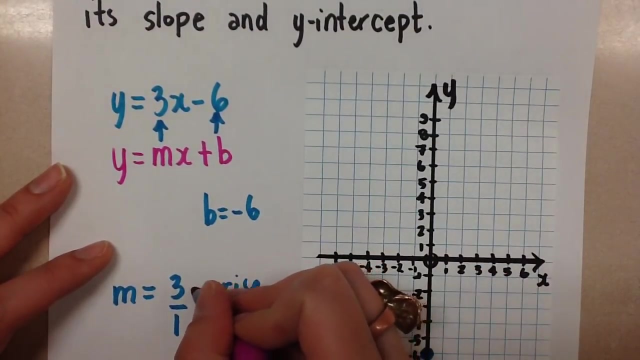 If you already had a fraction for your slope, then you would use the numerator of the fraction for the rise and the denominator for the run. But since we didn't have one, we're going to create that denominator. And now we see that the rise is positive 3 and the run is 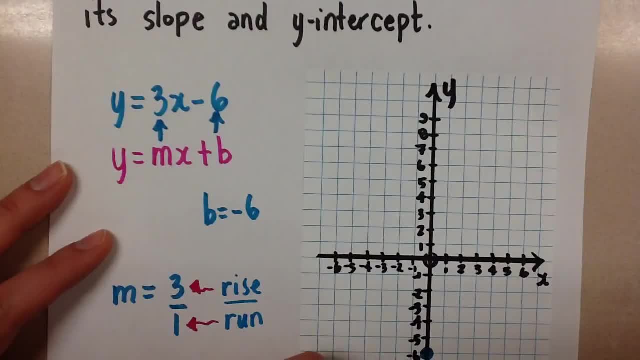 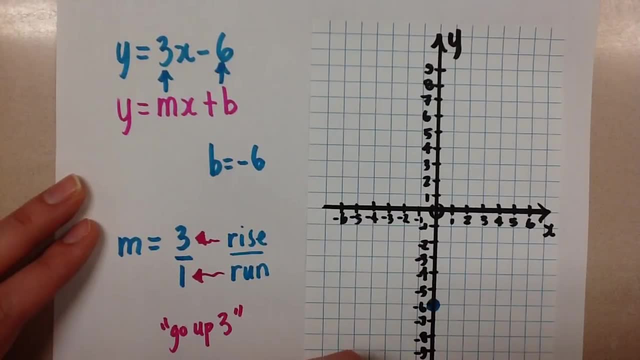 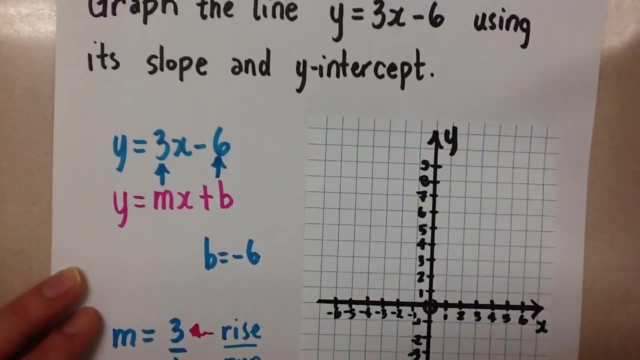 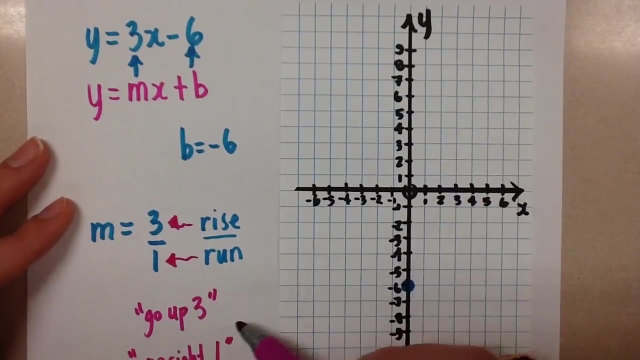 positive 1.. Go up 3 for the rise and go right 1 for the run. So we're going to go over to the y-intercept that we started on the graph here And we're going to do exactly what the rise tells us. Go up 3, because it was positive 3.. So from here I'm going to count: 1,, 2,, 3,, 4,, 5,, 6,, 7,, 8,, 9,, 10,, 11,, 12,, 13,, 14,, 15,, 16,, 17,, 18,, 19,. 20,, 21,, 22,, 23,, 24,, 25,, 26,, 27,, 28,, 29,, 30,, 31,, 32,, 33,, 34,, 34,, 35,, 36,, 37,, 38,, 38,, 38,, 39,. 39,, 40,, 40,, 41,, 42,, 43,, 45,, 47,, 48,, 46,, 49,, 50,, 51,, 52,, 53,, 49,, 51,, 52,, 52,, 53,, 54,, 55,. 56,, 57,, 56,, 58,, 57,, 52,, 56,, 59,, 52,, 53,, 57,, 59, upset. right now we're placed going up here. Let's do two points, one up and one down. 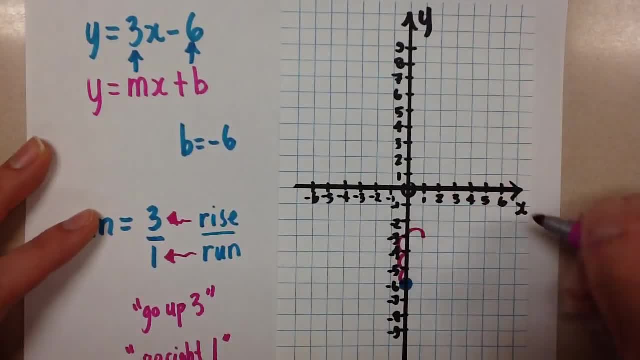 You're going to go 3 up, two points, Two points down, Three up, Two points down, Three up, Three up. Then I'm going to do what the run says, which is: go right 1, right 1.. Right there. 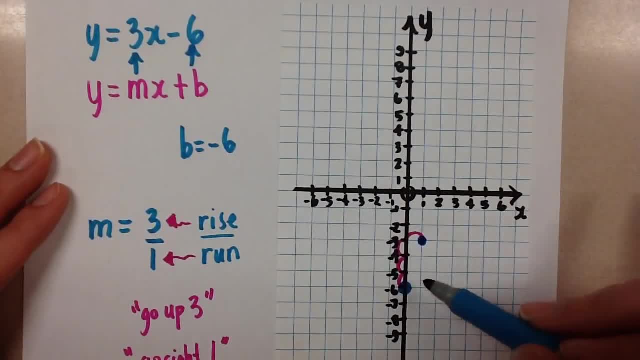 is my new point for this line. Right, there is my new point for this line. So now we have two points. Wait for me. So now we have two points, We can draw a line through those two points, points, and that's the line for this equation. I can also keep going with my slope if I want. 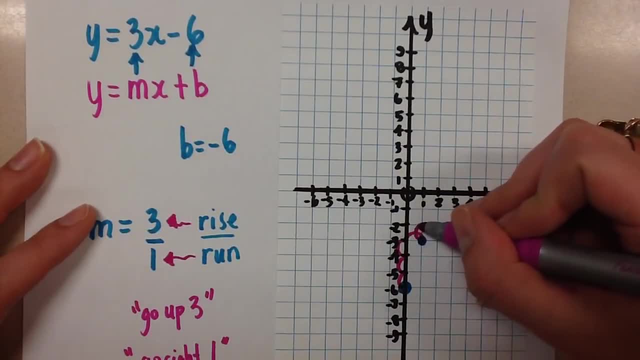 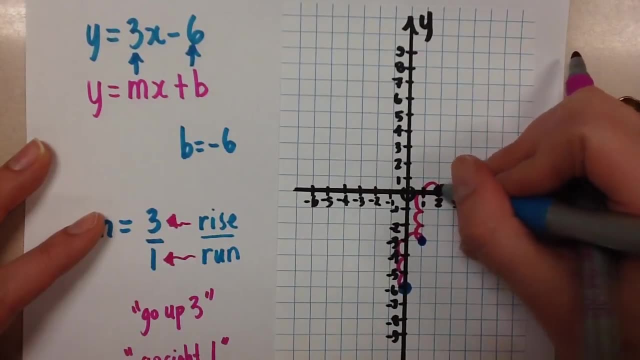 more points Again, I would go up 3, 1,, 2, 3, and right 1, and right there would be another point, And I can keep doing this until I get as many points as I want. but really you only. 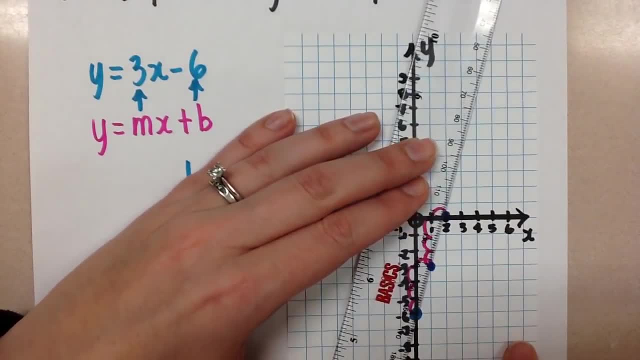 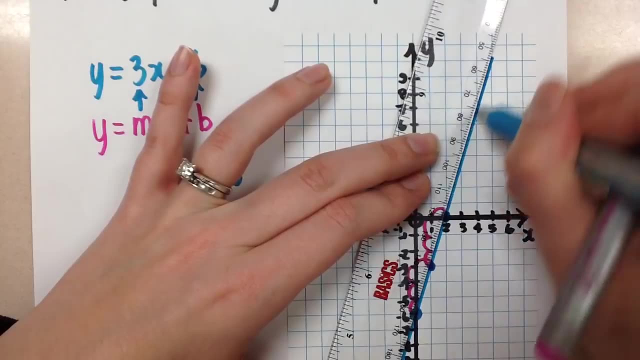 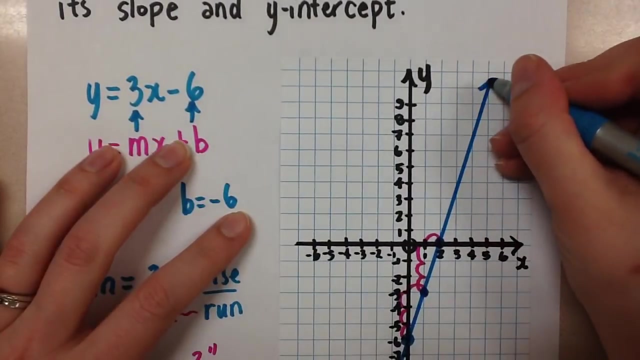 need 2 points to draw a line. So we take our ruler now and we try to line these up as best as possible. Draw your line all the way across the grid, nice and long. We'll put arrows because we know this line continues in both directions And we'll label this y. 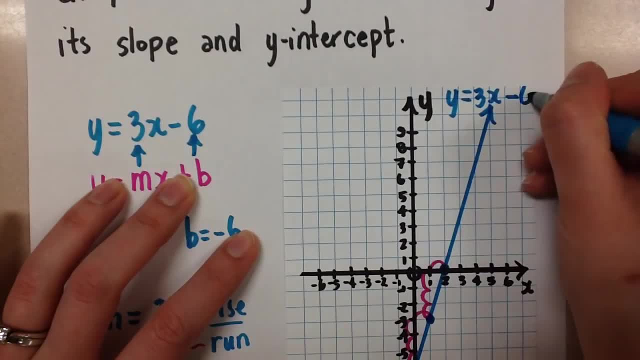 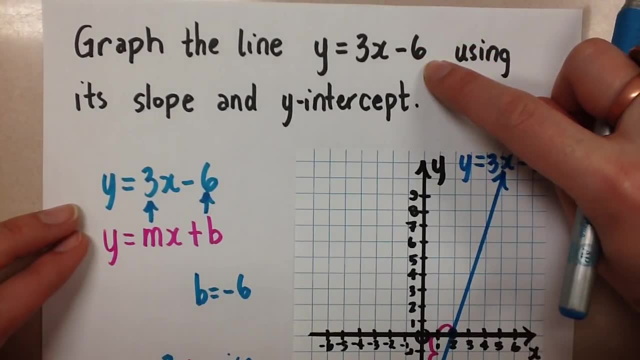 equals 3x minus 6.. And that is the graph for this line, given to us in slope y-intercept form. Thank you. Thanks for watching, Mrs A Loves Math. 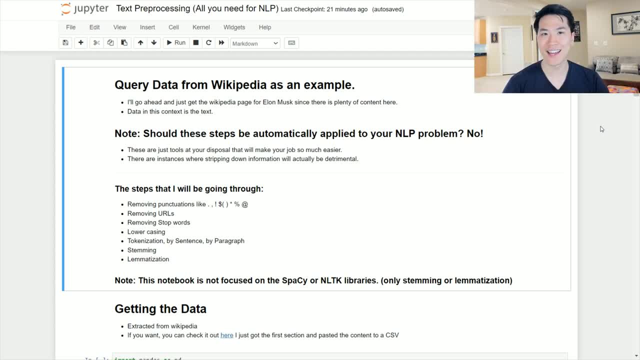 hey everyone, welcome back to my channel where i talk about all things tech and finance. in this video i'm just going to be going everything that you really need to know about the text pre-processing pipeline within the nlp framework, and you can apply these skills for more technical 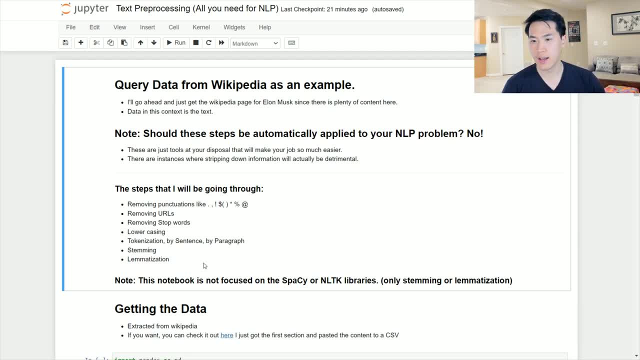 and more complex nlp type situations. so these are the general steps. i'll be going through punctuations, urls, stop words, lower casing, tokenization, stemming and elementization and throughout this entire notebook that i'll just be iterating through. i will primarily not really focus on the spaCy and nltk libraries, only when needed. 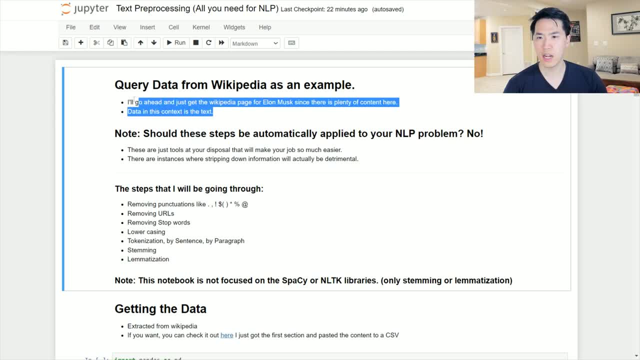 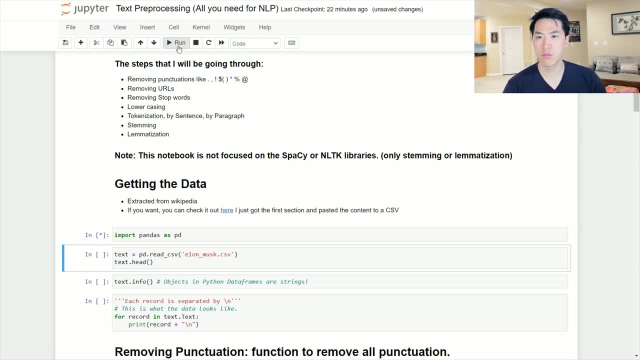 such as when i'm using stemming or elementization, and so the data i'll be using is from a wikipedia page. it's just like the page of elon musk, for instance, and we will see that over here, so let's go through and start iterating. this is the general text that we will be using. this is just a data. 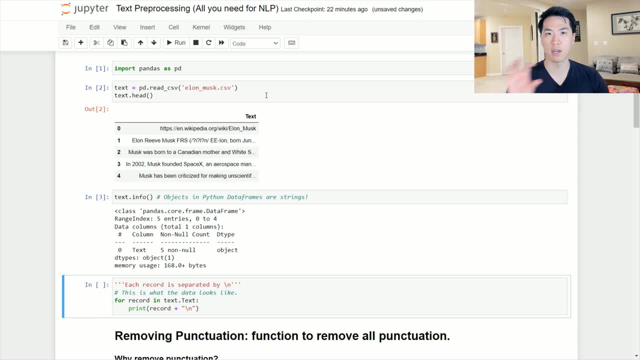 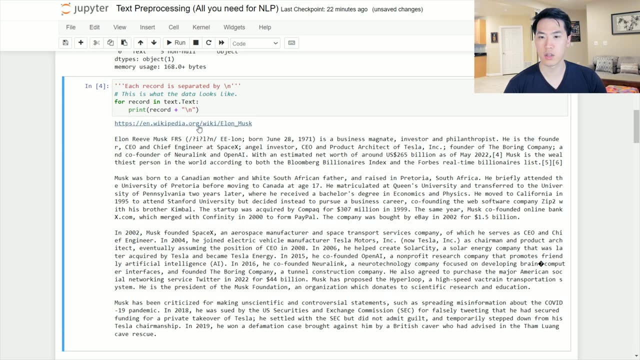 frame. so i essentially just copied paragraphs into each separate cell within the excel file and this is what it looks like. so this is the data we'll be going through. it's so far. first one is the link. you can go ahead and check that out. so these are the paragraphs we'll be 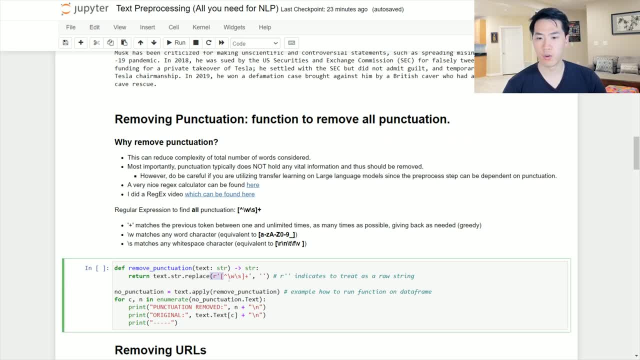 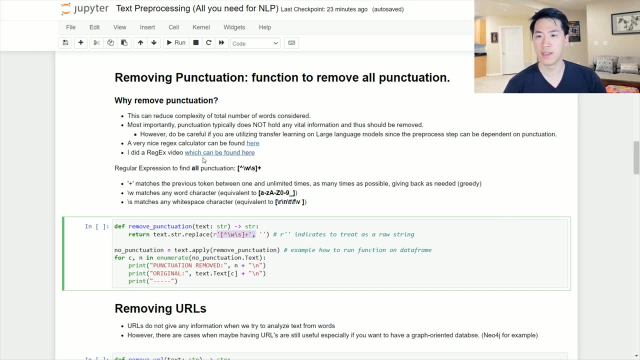 working with and this is going to be removing punctuation. so, for instance, when you're using the regex function, if you just want to remove all of your punctuation, this is just the regex string and i already did a regex video on that, so you can just go ahead and check that out. the link is in. 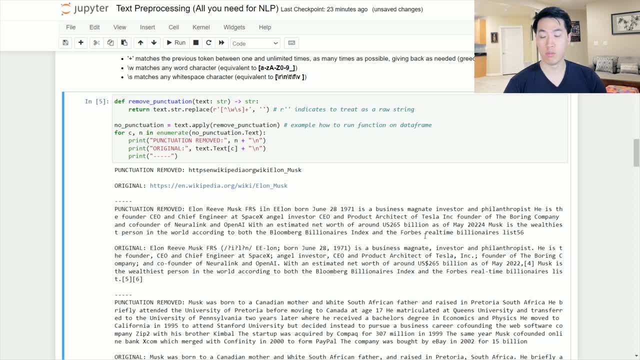 the notebook and also in the description below. this just goes ahead and remove all of our punctuation. so this is our original text and this is our cleaned text. you can automatically see which has been removed. you got those funny characters. you got the dollar signs that were removed, the brackets and so on and so forth.